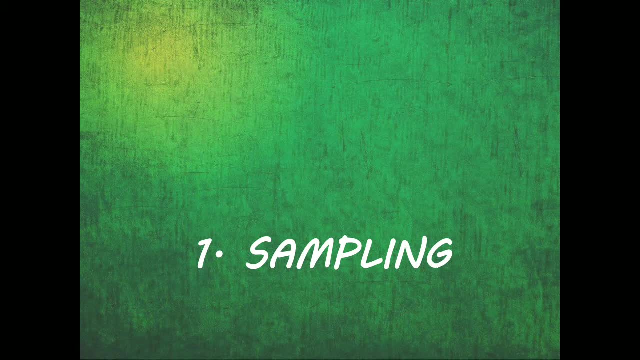 a representative of your entire population. So if you do not do it under aseptic conditions, you will get false results at the end. Hence, to make sure that you are taking the exact representative of the sample, you have to take the exact representative of the sample. 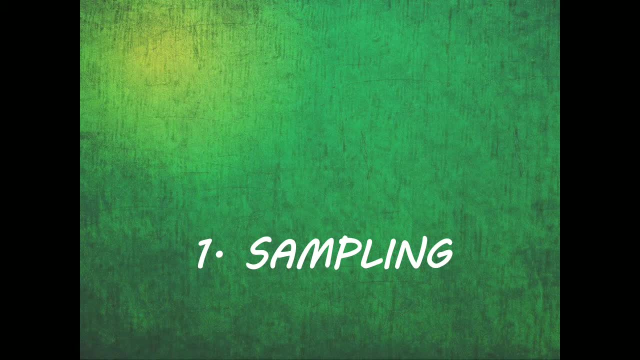 Say, I am looking for the population of algae that are growing in a water body. So if I need the exact representative, I need to make sure that I sample it perfectly. I sample it under complete aseptic conditions so that there is no other contamination, either from the air or from. 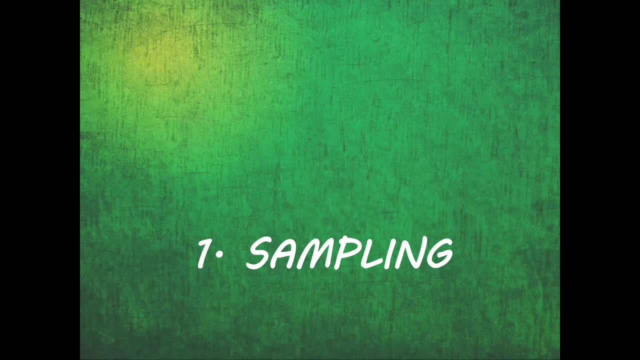 my hands, my mouth or by the way of my handling, from the soil There should be absolutely no contamination. Hence sampling is a crucial step. It is the first and the most crucial step to make sure that we are collecting the specimen under aseptic conditions. Now the method of sampling. 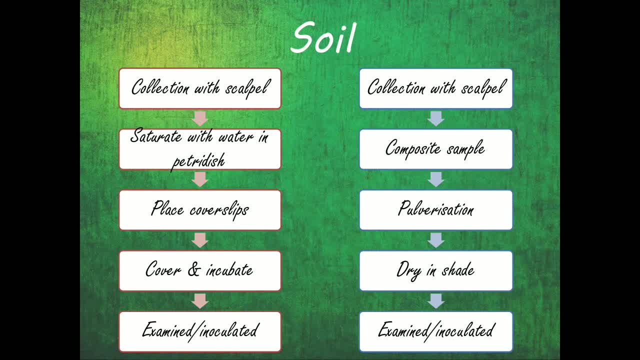 will differ whether you are looking into soil or water sample. So let us first see how do we collect a soil sample. Now, soil sample collection and processing can be done in two different ways. So the first method of collection and processing is we take an aseptic scalpel and, with the help of the 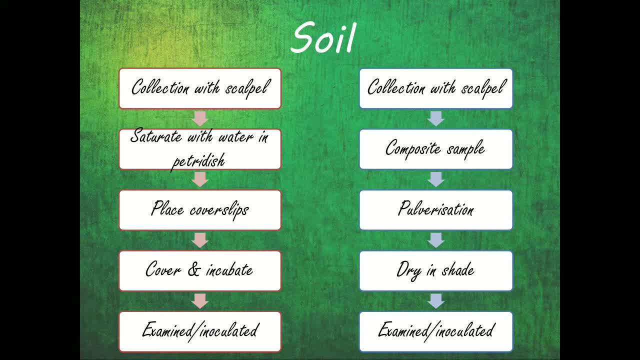 aseptic scalpel, we have to cut out or obtain an aseptic sample from the soil. So we have to cut out or obtain a surface soil or the surface layer, because usually algae are growing in the surface layers. So we obtain surface soil which is having a dimension of 30 centimeter into 30 centimeter. 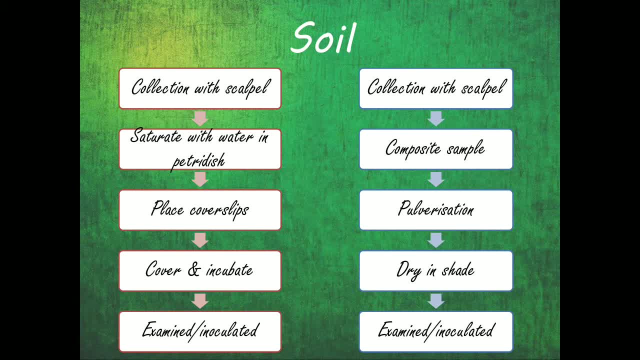 into 10 centimeter. This kind of surface layer is collected randomly with the help of a sterile sample or a very clean scalpel, and this can be collected from different sites. Now, once the block of soil is taken and it has been removed with the help of a, 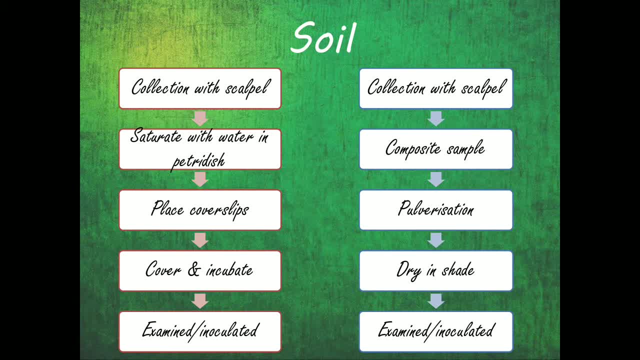 scalpel, then the method is going to differ. So collection of the soil with the help of scalpel remains same. After that, one method that can be followed is, after collecting the soil sample, the soil block can be kept in a petri dish and we can add enough water to saturate that soil block. 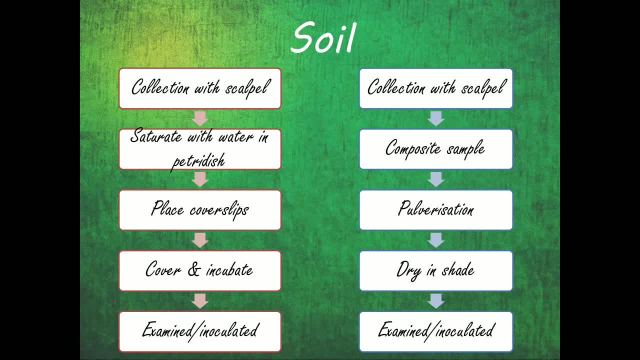 Once the soil block has been saturated with water, few cover slips are placed on top of the soil block and the dish is left open so that excess of the water can evaporate. Once the excess of water has evaporated, the petri dish is covered with its lid and incubated. 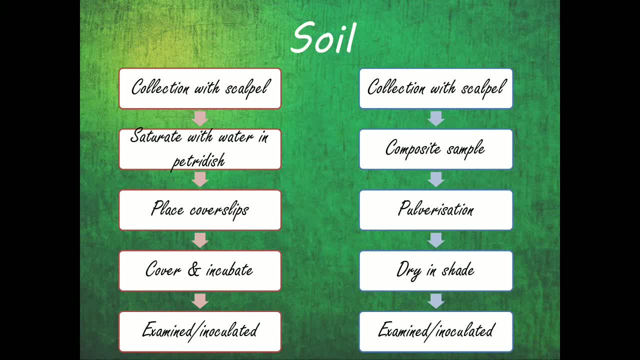 After a few days we will see that the young algae or the motile algae start multiplying, which can be either removed and examined or further inoculated into a medium aspera requirement. This is one method where we are going to take the soil block and assess the soil block directly by 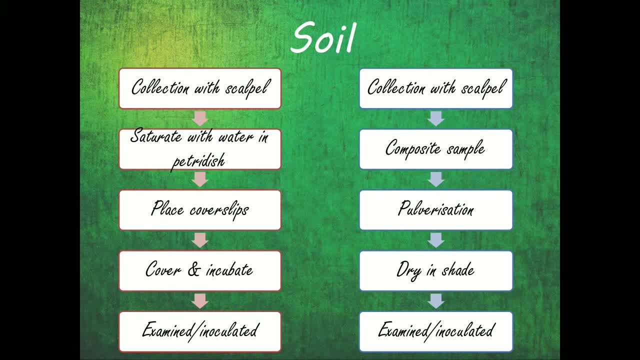 adding a little water. The second method is after collection of soil block. with the help of a scalpel the soil is converted into the block, is converted into a composite sample by mixing it thoroughly. So the soil is mixed thoroughly, converted into a composite or a mixed sample, and then pulverized or 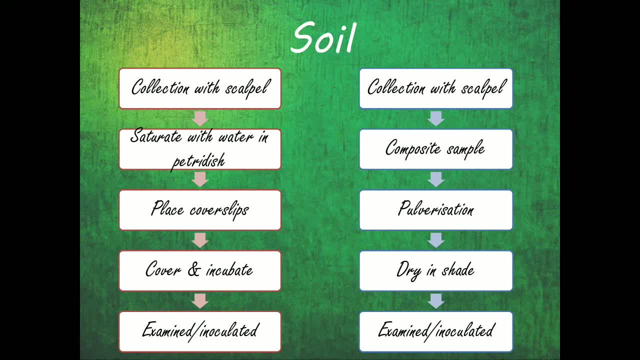 broken into very tiny pieces After pulverization, it is dried in shade and then it can again either be examined directly or it can be inoculated into a different medium. So here we allow the organism to grow, after which it is examined Here, instead of allowing it to grow. 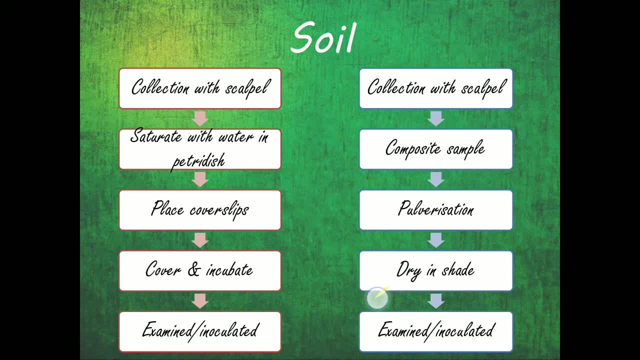 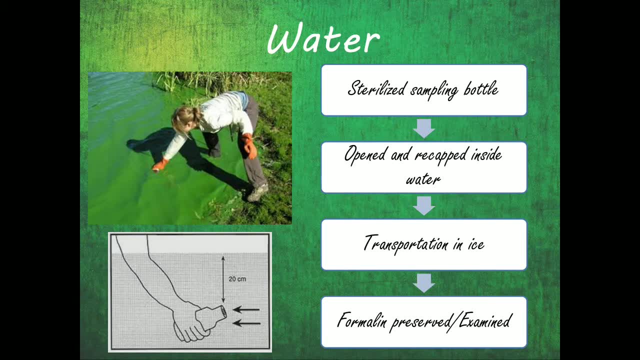 we are mixing it thoroughly and then drying it and then processing it. These are two methods by which we can process soil samples. For a water sample, we need to make sure that always a sterilized sampling bottle is taken, like how we had used a sterile scalpel in case of soil sample. 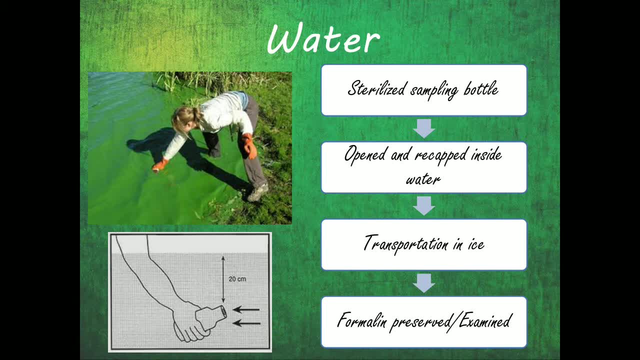 Here we need to use a sterilized sampling bottle. It has to be taken care that the bottle is lowered into the water body and only then opened, So the bottle should be opened and recapped inside the water. The sterile bottle has to be lowered into the water body at a depth. 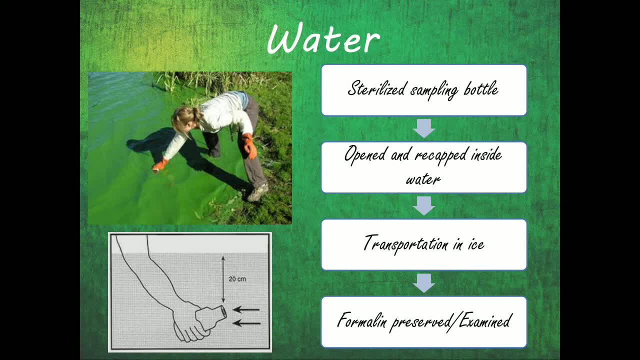 where we want to obtain the algal sample, After which it is opened, water is collected and then it has to be recapped within the water itself. This bottle can be then transported in ice and further either examined, or we can go ahead with preservation in formalin if we don't want to grow. 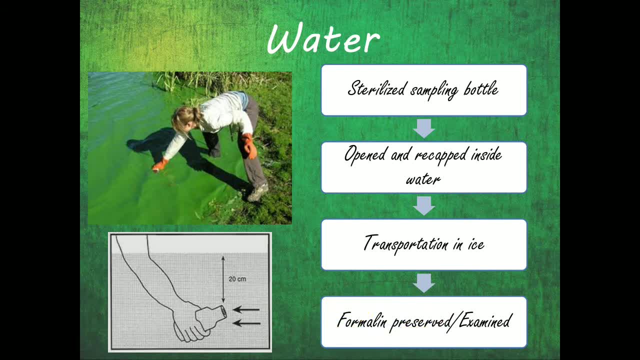 the particular algal sample. Now, if it is a benthic algae, that is, an algal sample which is present at the bottom of a particular water body, then we need to scrape out the sample from there and then that can be used for processing. So the first step is collection of the specimen or the sample in an 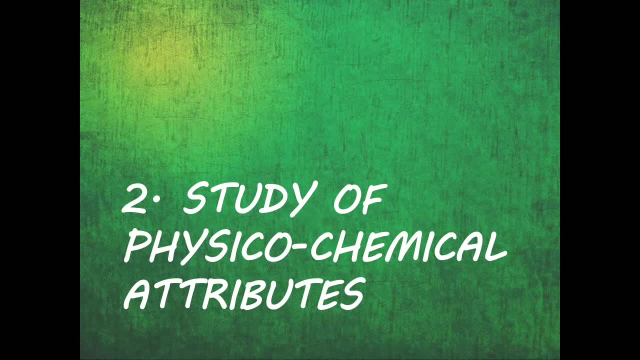 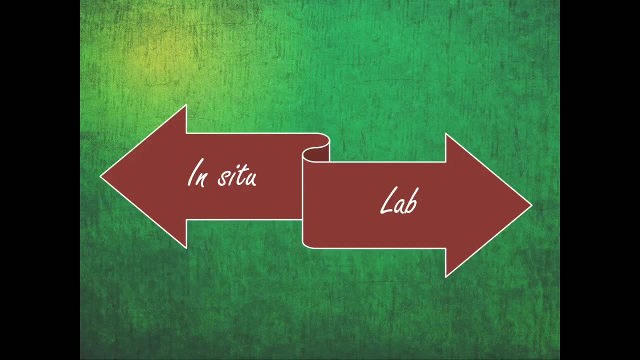 aseptic condition. that is called a sampling. We move on to the next step, that is, the study of physicochemical attributes, or physicochemical parameters or characters. Now these can be done either in the lab and or it can be done in situ. Actually, it's not either. we need to do both. So 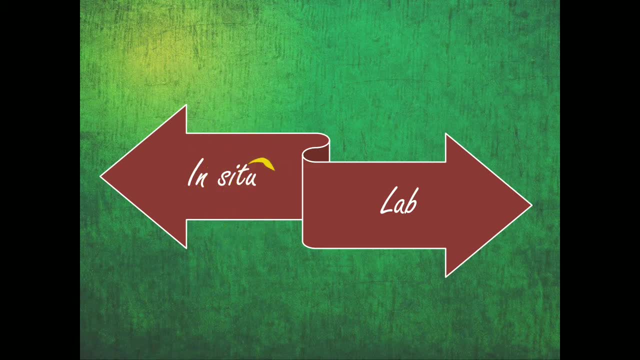 in situ studies or on-site studies include the checking of temperature and moisture if it is a soil sample, So a soil thermometer or a soil moisture meter can be used for checking the temperature and moisture, respectively at the site of sampling And if we are using a water sample. 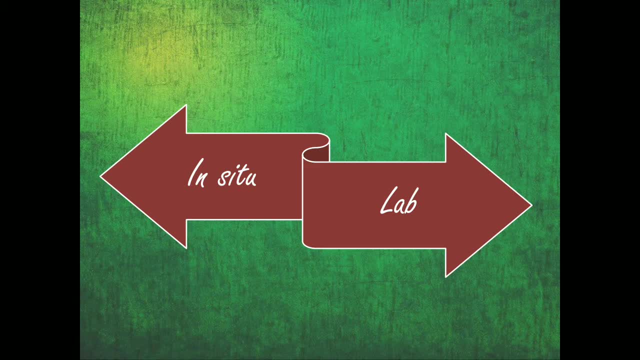 only the temperature of the water sample need to be checked on site. Those are the in situ studies that need to be done In the lab. the different parameters that need to be checked are the pH, which can be of the water sample, or the temperature of the water sample. So in situ studies we need to. 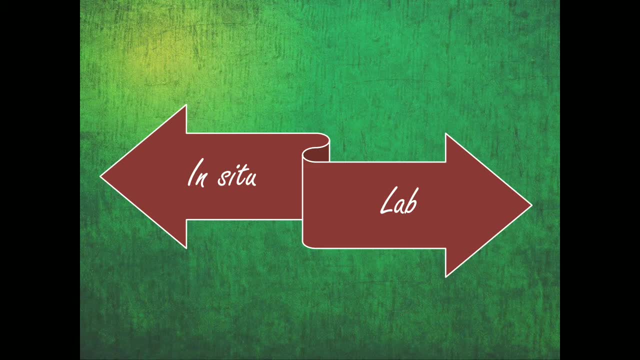 check the pH, or if it is a soil sample, it has to be suspended in distilled water and then the pH has to be checked. Electrical conductivity has to be checked with the help of a conductivity meter, The total nitrogen and the available phosphorus and organic carbon that is present in that sample. 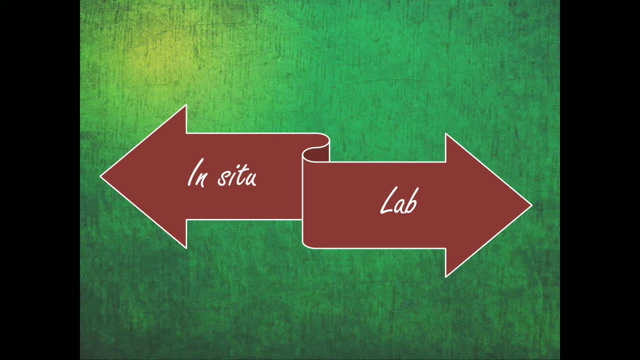 needs to be checked. And finally we need to look for the water soluble cations with the help of a flame photometer. So in the lab also there are a few studies that need to be done before we get into processing and study of the sample. 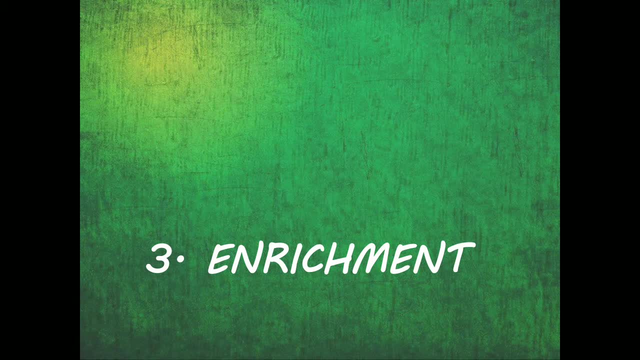 The third step. again, this is a very, very crucial and important step in any isolation technique, that is, enrichment. Enrichment is where we are enriching the sample, or we are making sure that the algae that is present in the sample is growing proliferatively in our lab. So we might have taken 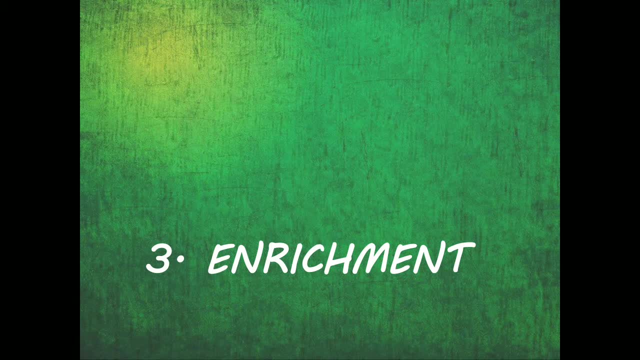 a sample, a representative sample, which will have a very small quantity of the algae, But I want that algae to grow more. What we do here is we take the sample and we add some excrement to it And we add extra nutrients to it. The moment we add extra nutrients, the algae which might be in very 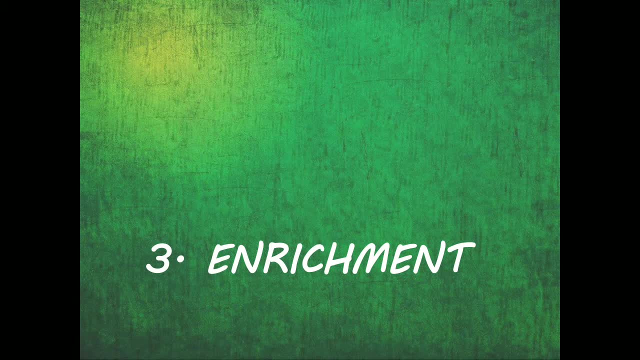 low numbers will start growing rapidly and will give us more volume or it will give us more number of our particular desired algae. So enrichment is very, very important before we get into actual isolation or colony formation or any other studies, because we have to increase or bulk up the number. 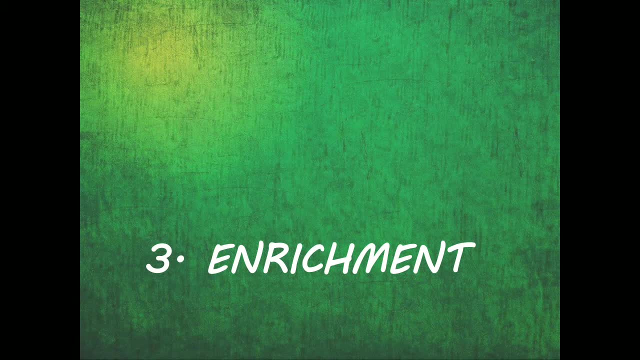 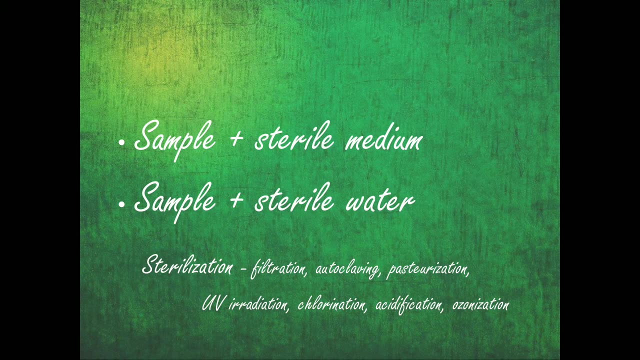 of organisms, or we have to increase the microbial load in our sample, And that process is called as enrichment. So for enrichment of algae we have to take the sample that has been collected aseptically and mix it either with sterile medium or with sterile water. Now when? 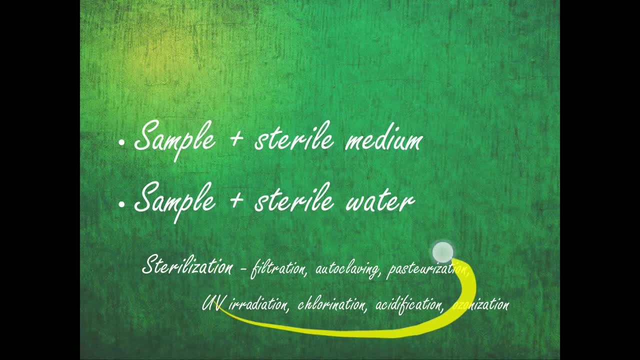 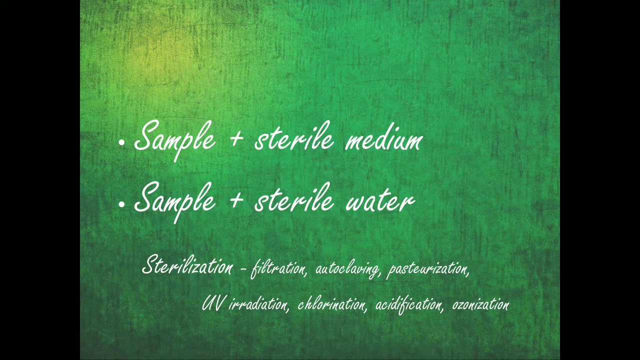 we say sterile medium or water. the sterilization can be done by various physical and chemical methods. Physical methods include filtration or autoclaving or pasteurization or UV irradiation, And the chemical methods include chlorination, acidification and ozonization- Usually sterilization. 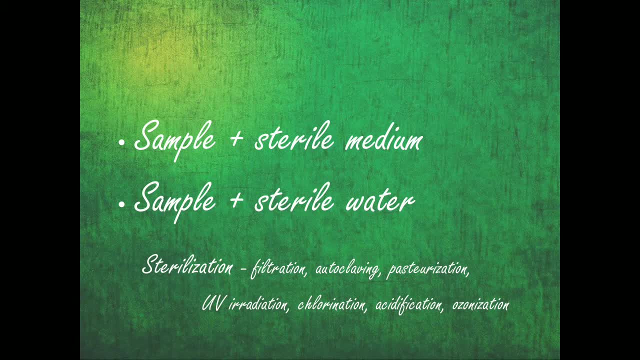 is preferentially done by physical methods of autoclaving and pasteurization. They are the most preferred because they are effective and economical both. So once the sample has been mixed with the sterile water or the sterile medium, it is shaken vigorously and the algae 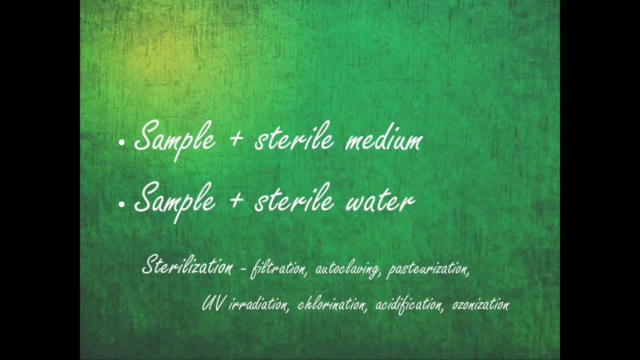 are picked up and transferred into a medium. Again, the process is repeated so that maximum number of algal cells are dislodged. So the sample, once it has been mixed with the medium or water, is shaken vigorously and the algae are picked up and transferred into a medium. 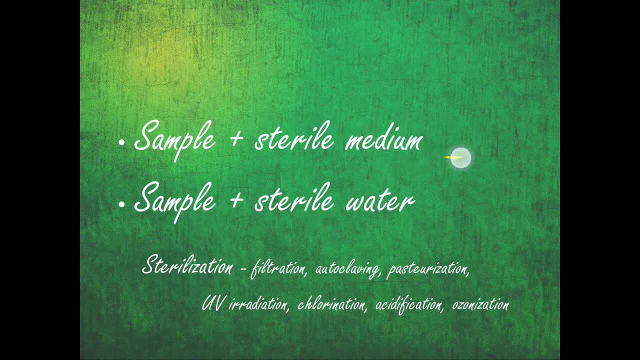 The process is repeated. the shaking process is repeated so that algae can be separated completely. The medium that we use can be with or without a nitrogen source, based on whether our algae is nitrogen fixing or not. If our algae cannot fix nitrogen, there is 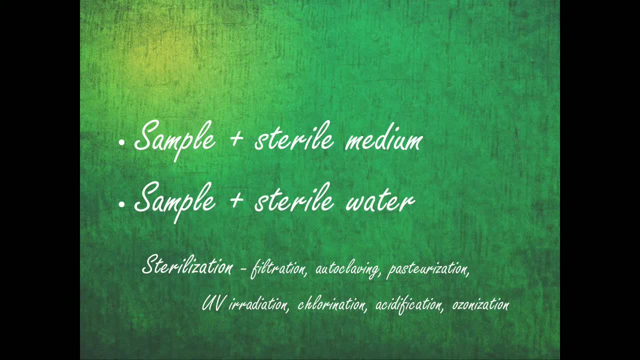 no point of removing the nitrogen source. then we have to give a nitrogen source. So the medium again depends on what kind of algae we are looking for, And the culture of the soil is different. The culture of the soil depends on what kind of algae we are looking for. So the culture is after mixing it with these sterile medium. 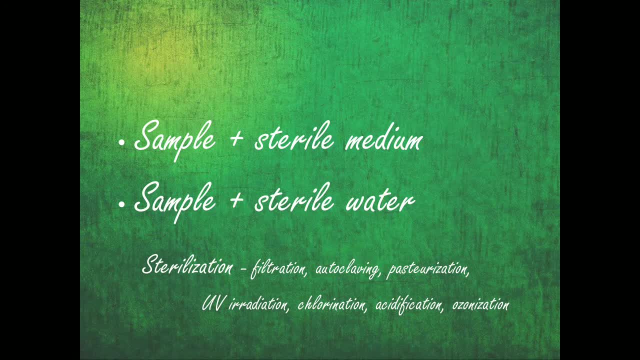 or water, and shaking vigorously, we transfer it onto a fresh medium and then the culture is kept at an illumination of maximum 3200 lux, but it depends on what kind of algae you are growing, And the intensity of the light has to be maintained with either using natural 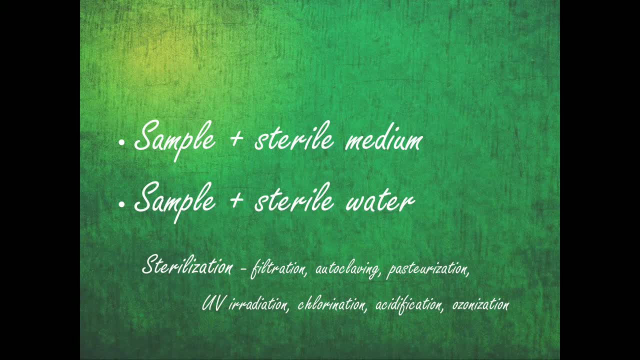 source or by using white fluorescent lamps, So the desired algae is allowed to grow and then it is picked up and transferred into a medium. So the culture is: after mixing it with these sterile medium or water and shaking vigorously, we transfer it onto a fresh medium. 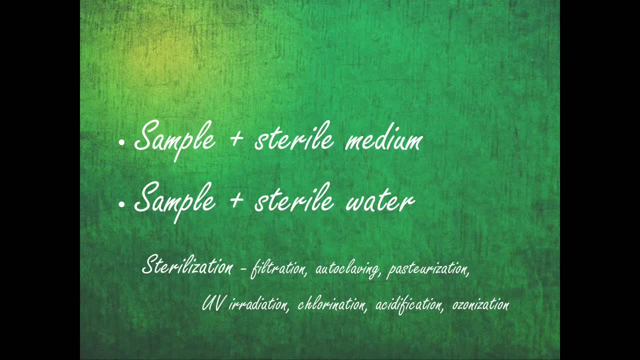 After mixing it with these sterile medium or water and shaking vigorously, we transfer it onto a solid medium. So enrichment is usually done in a liquid medium, such that the volume of algae we obtain is more, after which it is transferred onto a solid medium. The next process is once we see that the algae has started growing in the broth or in the 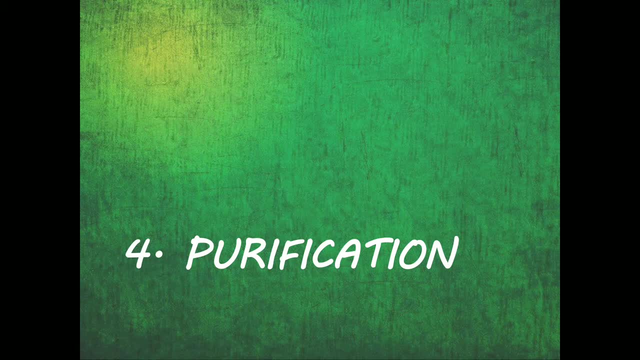 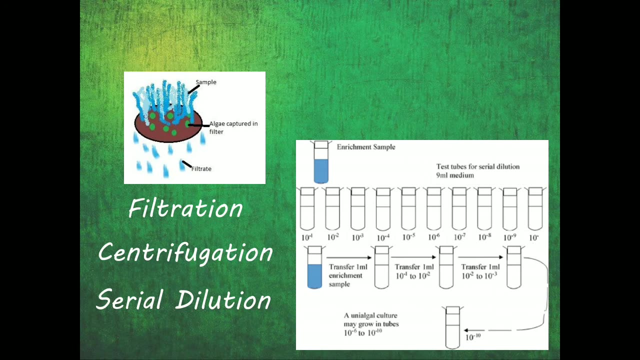 liquid culture that we have provided. it needs to be purified from there, because along with algae there will be many other organisms and we want only a unialgal culture. The purification can be done by simple techniques of filtration or sanitization, So we have to purify the 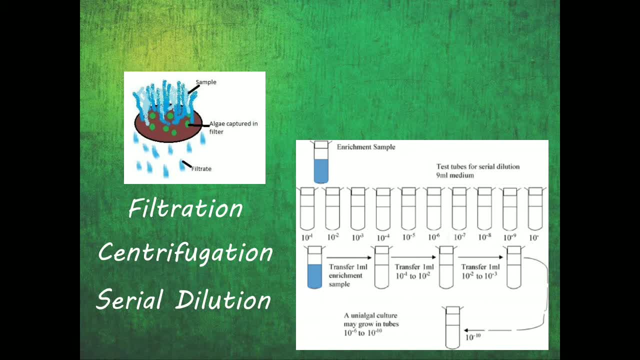 or centrifugation or serial dilution. These are the basic techniques that are used. They are the techniques which have been used from a beginning and they are done to obtain unialgal cultures, that is, obtaining only one kind of algae. But in some cases we would need 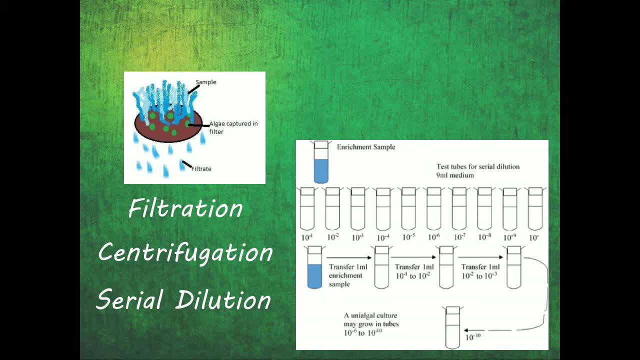 an axenic culture. Axenic culture is wherein the culture should contain only one type of alga and no bacteria or fungi or protozoa, Whereas in a unialgal culture, though we have only one algal population, there may be the presence of bacteria, fungi and protozoa. So when we want, 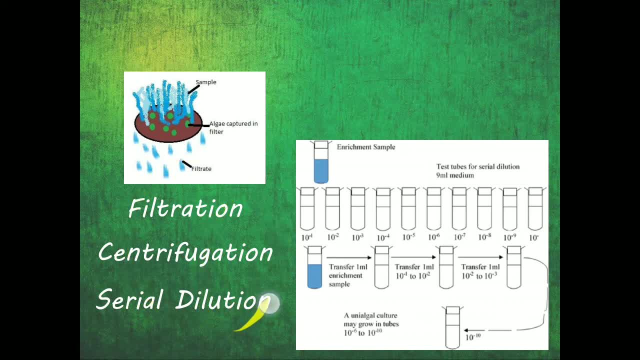 to go for unialgal culture, these techniques will suffice. but if we want to go for an axenic cultures, then the techniques that I am going to tell after this, they will have to be used A little more advanced techniques would have to be used Usually when we want to go for 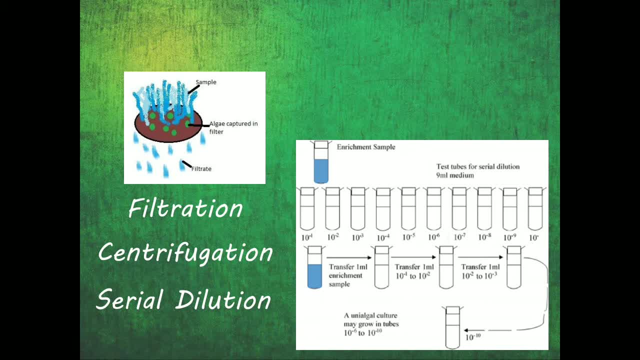 purification it. Sometimes it is necessary for us to add antibiotics or antibiotic treatment has to be done. For example, we could add penicillin or streptomycin or gentamicin- any of these common antibiotics. if we use in the microalgal culture then it will diminish or reduce the bacterial growth without 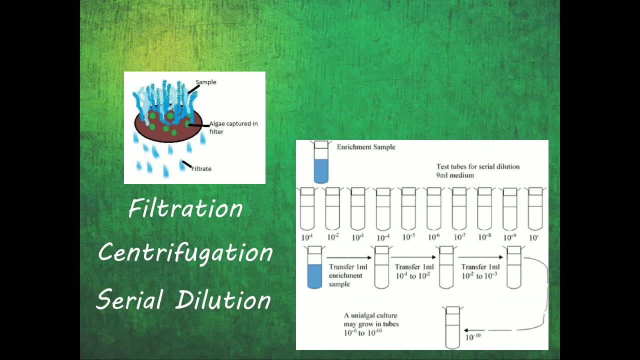 affecting our algal growth. But in case of axenic cultures we not only antibiotic treatment, we may also have to go for treating the sample that we obtain after filtration or centrifugation or serial dilution. post-treatment, We might have to go for one more round of washing, or extensive washing may need to be. 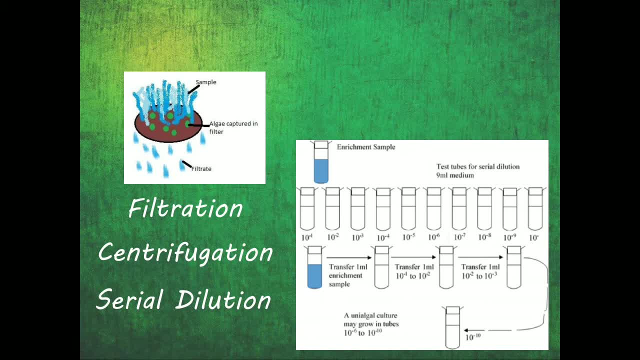 done, We may have to add antibiotics or if there are resistant stages, such as zygote or echinetes of algae, they can be treated with bleach so that the other organisms and epiphytes can be killed and only these pores will germinate and we can use them. So basically, 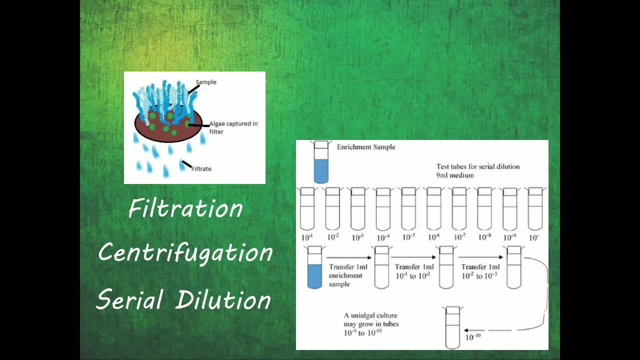 it is necessary for us to try out different concentrations of bleach or different times of exposure, Different techniques, to find a solution. So, basically, it is necessary for us to try out different concentrations of bleach or echinetes of algae to find a treatment that will ultimately kill all the other organisms. 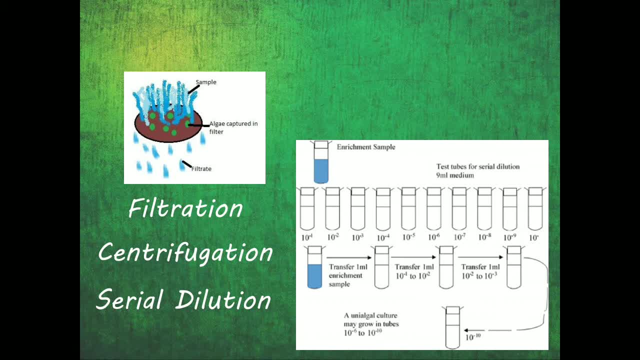 but not our algae of choice, The type of treatment. everything is based on the algae we are going to work with. So filtration is the simplest, wherein a membrane filter is used. The filter could be made of cellulose acetate or polyamide or colloidal membrane or teflon membrane, polypropylene. 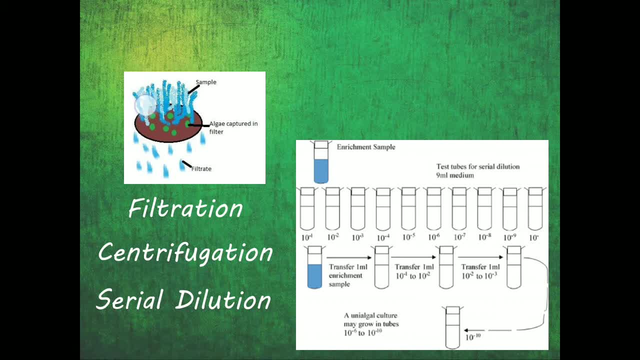 These are the membranes that are used and the algae is passed through the filter, The culture that we have allowed for embridging. So this is what we are going to do. We are going to go through the process. We are going to go through the process. We are going to. 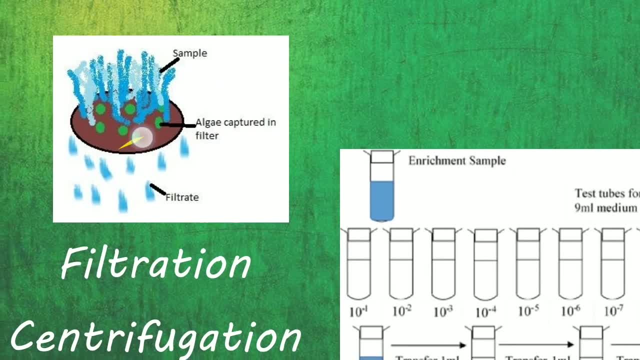 take the filter, We are going to pass a liquid or a strain on the filter. We are going to pass a filter to filter this liquid or a strain. So the liquid is passed through the filter, The algae are captured on the filter and we. 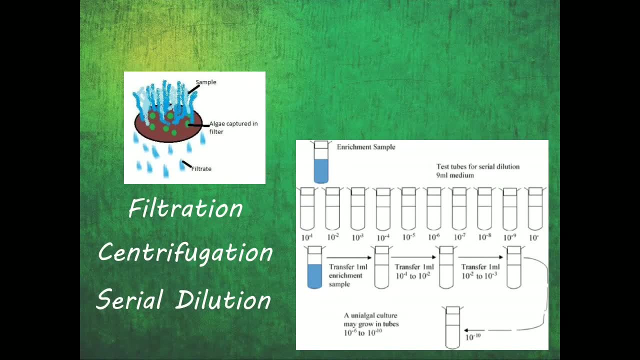 get our filter in at the bottom, So the algae are taken from the filter and transferred on to a solid medium. The second one is centrifugation, or it is also called as differential centrifugation or centrifuge washing, where multiple rounds of centrifugation are done to concentrate the 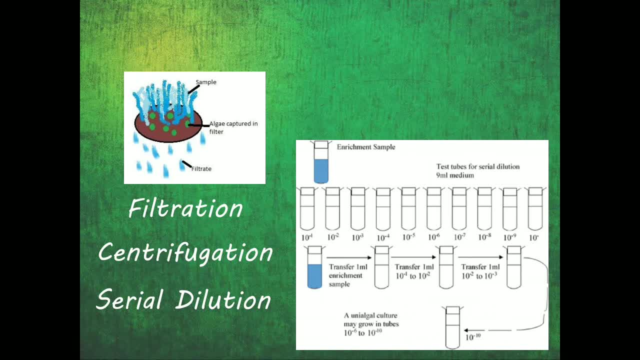 cells. So if we centrifuge at 3000 RPM for 15 minutes, we get a pellet. that pellet is our algae. The pellet is suspended in fresh water and homogenized again, So we can simply transfer it into the cell. So that is something that we can be clear We are going to use. 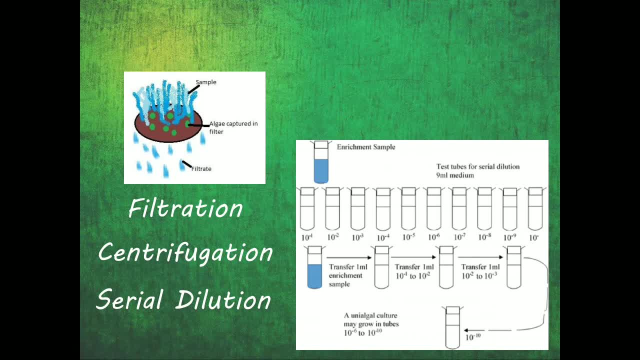 theculin here. in the next video We will be going to see how to do this. So let us see the again. centrifuge repeated. it is repeated two or three times and from every tube where we are suspending the pellet a streak has is done on an agar plate, so it makes sure that we get isolated. 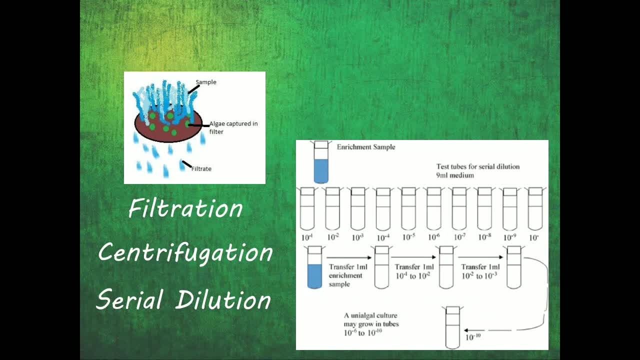 colonies or we get uni-algal culture. so this is also a very good technique. that is, centrifugal washing or centrifugation, or another one of the classic techniques is serial dilution, wherein we take the algal sample and in this case i have shown you a tenfold dilution. we could also do a. 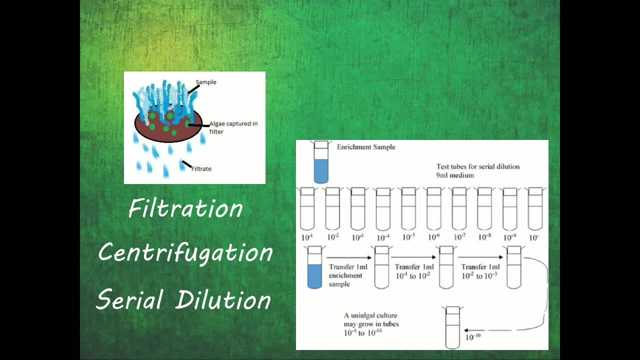 double dilution, so serial dilution, is wherein from the first sample, that is, the enrichment sample, we transfer on to the first tube containing nine ml of either saline or media or distilled water, and from there we progressively keep diluting. this is known as serial dilution, if you want to. 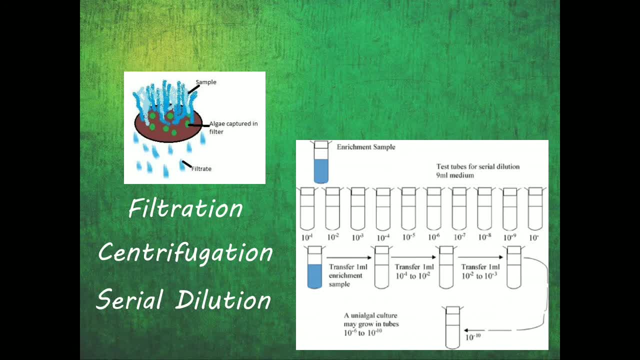 know more about serial dilution, you can always see another video which i have uploaded regarding serial dilution. so at the end of it we get diluted sample, the numbers of algae keep reducing and we get a double dilution. so serial dilution is wherein, from the first sample, that is. 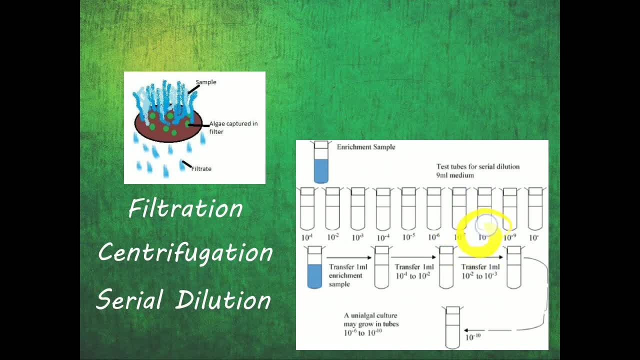 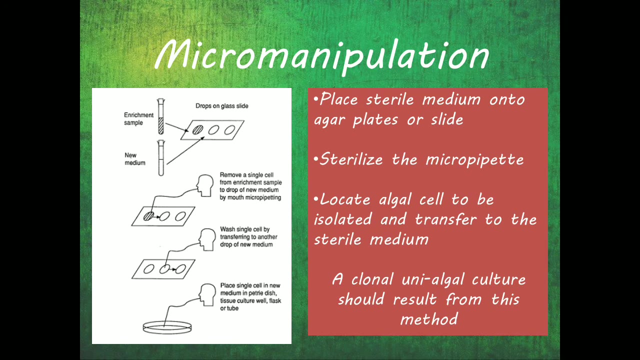 using and finally, towards the higher dilutions when we transfer them onto an agar medium, usually we will get a uni-algal culture. so these are some of the basic techniques which can be used for purification of the algae from the enrichment sample. the other more advanced techniques which 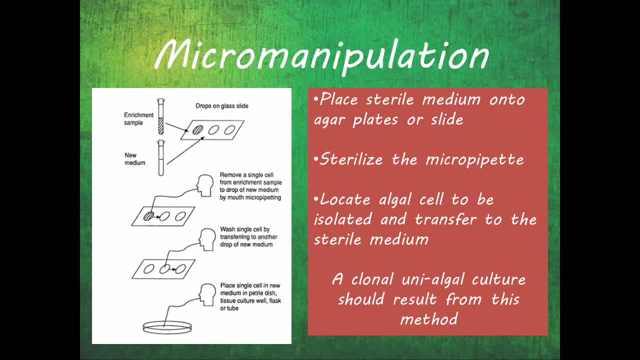 can be used to get axenic cultures are micromanipulation. now, in this case, micromanipulation is also called as capillary pipette aspiration. so in this case a capillary pipette aspiration is a capillary tube is converted into two micropipettes by drawing out and over a bunsen. 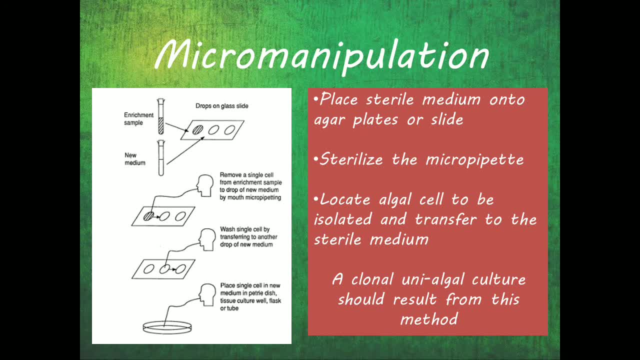 burner, so it is held on both the ends to form two micropipettes. these are. these micropipettes are different from the micropipettes used in rdt. now the micropipettes are made sure that they are sterilized, after which sterile medium is placed onto either agar plate or on a slime. 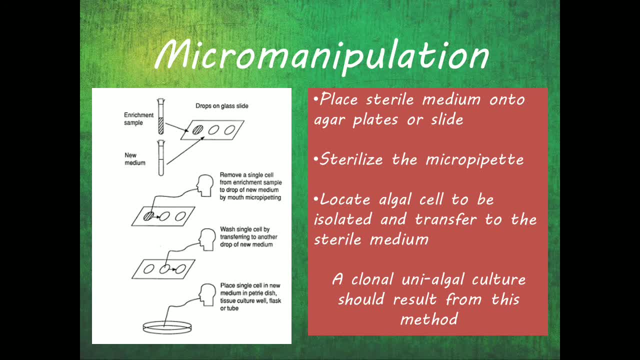 now the sterilized micropipettes are taken and with the help of that, the algal cell which needs to be transferred or which needs to be isolated is located. once the algal cell has been located, or once we have located which culture we want to transfer, 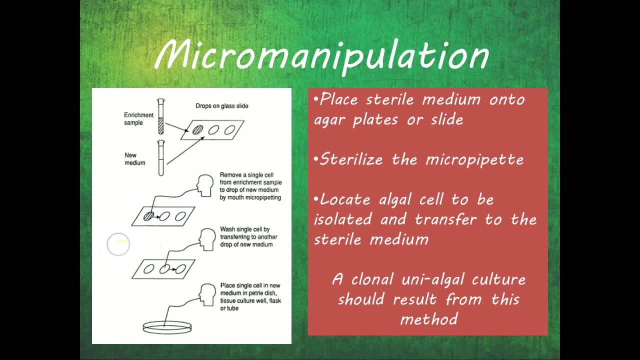 it is transferred with the help of the micro pipette onto the first drop or onto the sterile medium. after it has been placed on the sterile medium, which is in the plate or the glass slide, again the micropipette is sterilized with the help of hot water, and then the process is repeated. 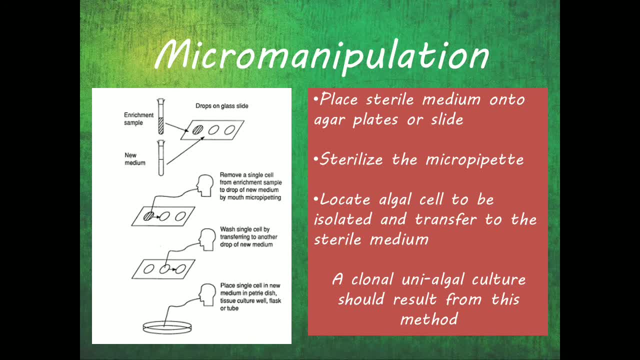 it is basically like washing the cell, so the, the culture which was placed on the first drop is then washed, where it is transferred into the next petri dish or into the next drop. from there it is transferred to the next petri dish. so in this way, 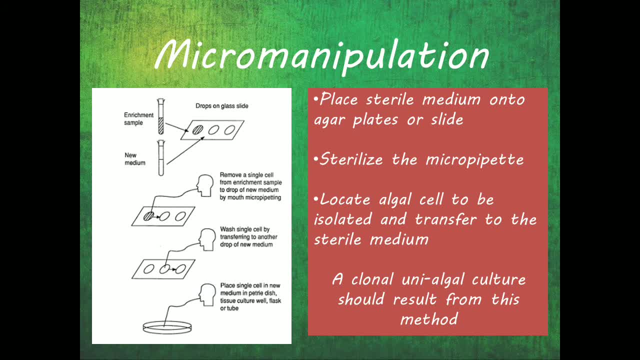 we are continuously transferring or washing the cell. more number of times we wash the cell, less likely is the bacterial contamination. we will not have much contamination happening because we are washing it. of course there is risk of damage with more number of times we are handling the cell. 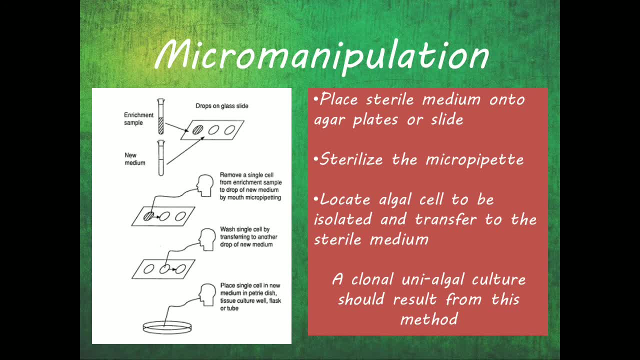 but then an optimum number of wash can be decided based on what type of algae we have. so we place, we keep transferring it and ultimately the cell is transferred into a dilute medium which is kept in a culture tube, or it could be kept in a petri plate. this culture vessel is then kept at an 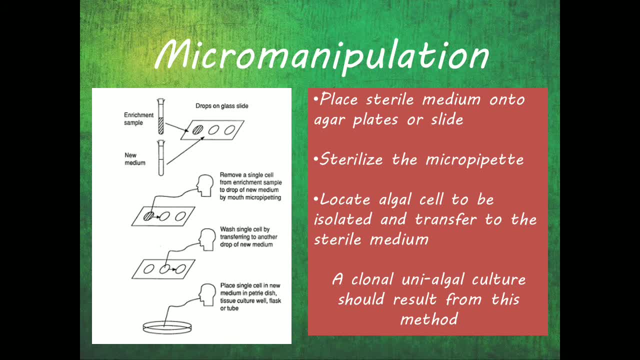 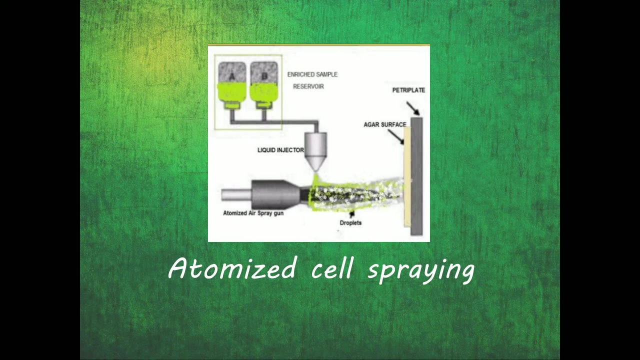 appropriate light, condition and temperature, and then after three to four weeks we can find the unialgal culture growing. so this is also a very easy method of micro manipulation. we then have at a time to use a randomized cell spraying or spraying technique. now, in this technique a 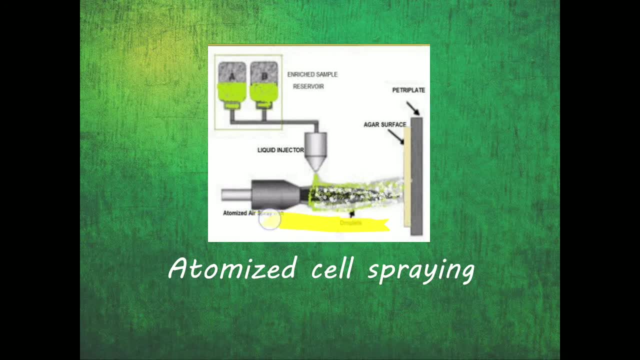 stream of compressed air is used. this is the stream of compressed air that is coming that is used to disperse the algal cells which are transferred through this injector. so the algal cells from the enrichment sample are transferred through the injector and at the same time there 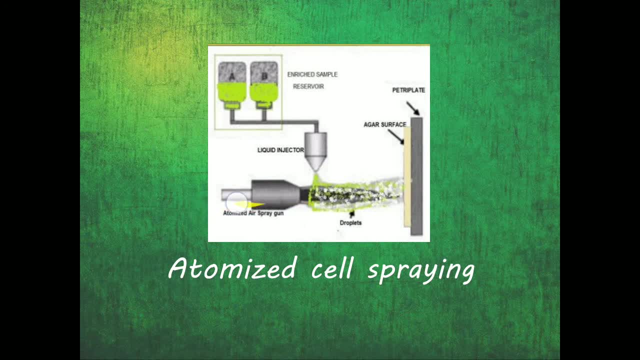 is a compressed air stream that is being transferred onto this mixture. when the air stream is being transferred through this mixture, it sprays the stream, it sprays this entire sample and that spray is landing on a petri plate which contains a solid medium, an agar medium. now, 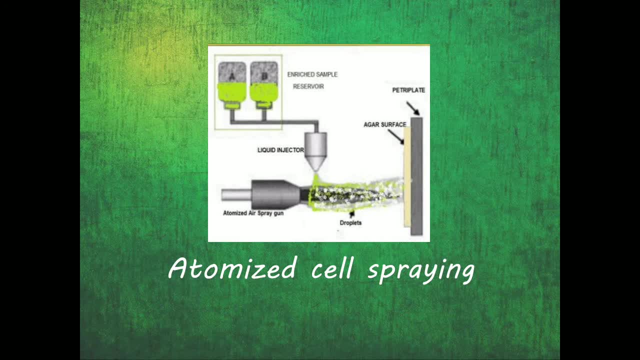 what happens here is when the spray is the airflow that is spraying, the suspended algae is being intercepted by the agar plate. so now, on the agar plate, instead of streaking, we have sprayed the culture, or we have sprayed the sample, which helps us to get isolated colony. so this is also 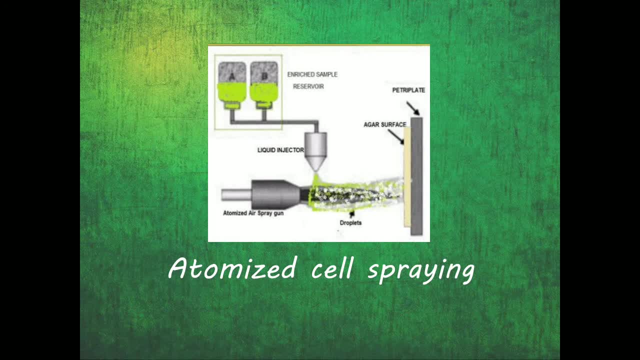 also a very good technique for obtaining isolated colonies of purifying the mixed culture or the enrichment sample into a unialgal culture. We also have other methods, such as flow cyprometry or automation. they are automatic isolation methods where what happens is again the cells. 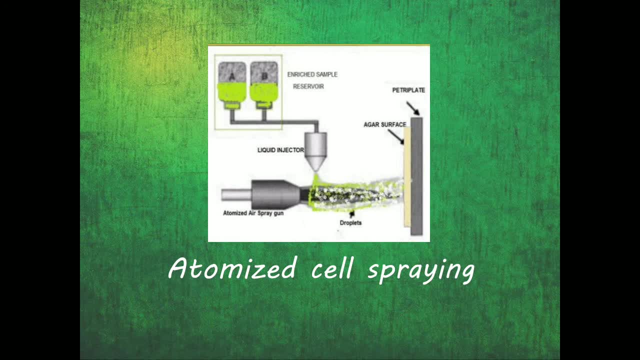 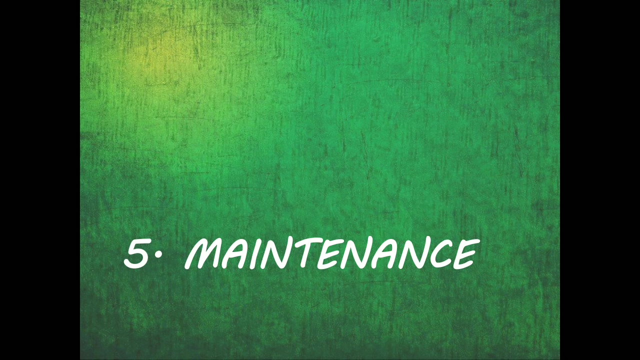 individual cells are being transferred and that is being collected and transferred onto a medium. So these are some of the methods that are used for purification of algal cultures. After the cells are purified or after we have obtained from the enrichment culture, we have obtained isolated cultures or unialgal cultures. they need to be now maintained. Now the maintaining. 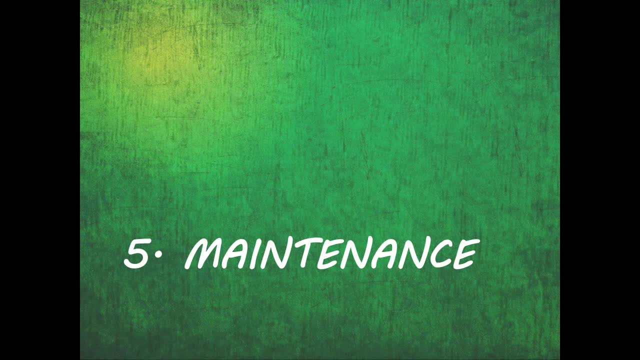 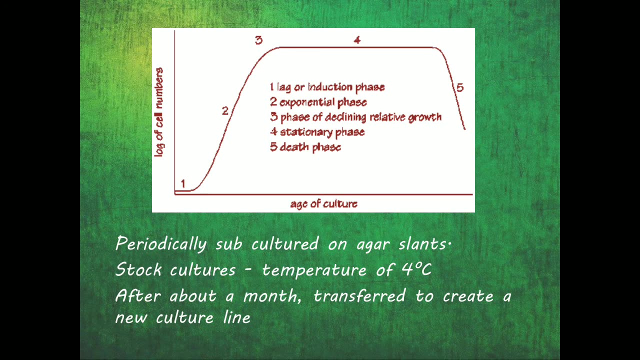 is done at different temperatures and different light intensities based on what type of organism we are working with. So usually for maintenance, we tend to pick up the organism And subculture it periodically onto agar slants. Now the picking up and subculturing is done at. 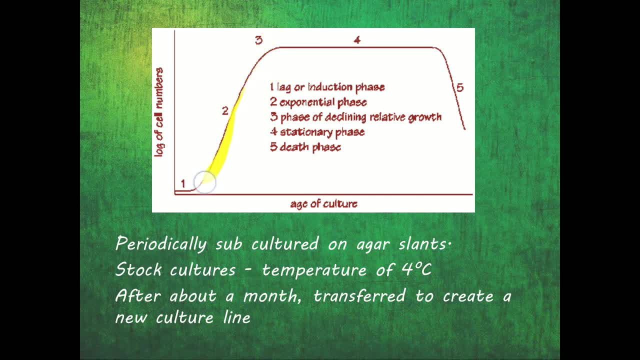 this phase at the decline phase, where the log phase or the active growth phase is ending, and before it gets into the stationary phase. usually the algae are picked up and subcultured onto an agar slant. After they are subcultured, they are stored. these stock cultures are stored at a 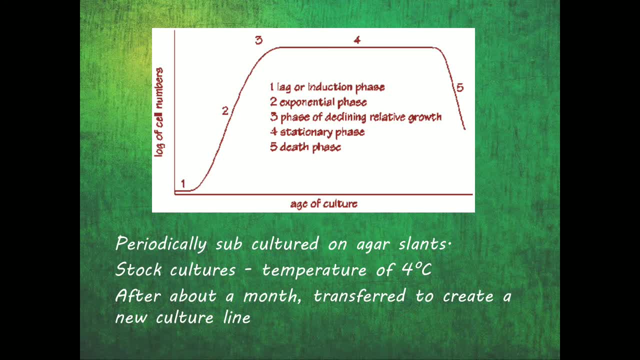 temperature of 4 degree Celsius. If the algae has been stored at a temperature of 4 degrees Celsius, it can also be stored at a temperature of 16 to 18 degree Celsius, but usually if it is in a broth culture, these broth cultures are stored at a temperature of 4 degree Celsius and then 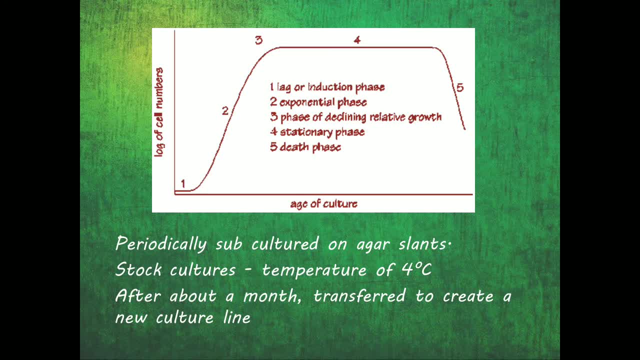 periodically subcultured. One thing to remember here is that the temperature is usually kept low so that the algae are surviving but they do not start multiplying, and the light source is a mix of white and warm white fluorescent lamps, So it makes sure that there is cool and hot both. 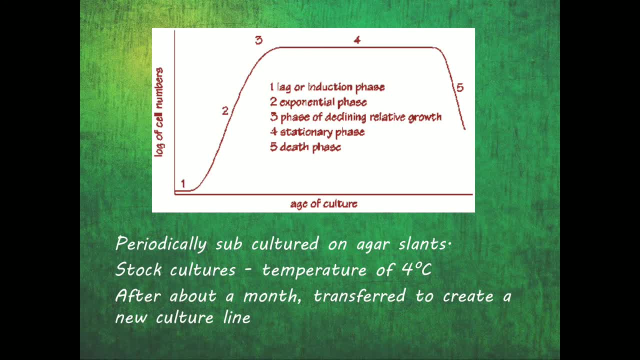 when we are trying to store the algae. Additionally, there are some algae which cannot be placed under bright lights, For example, if they are colorless strains of euglenoids, or even some green algae like polytoma or prototheca, or some other algae such as. 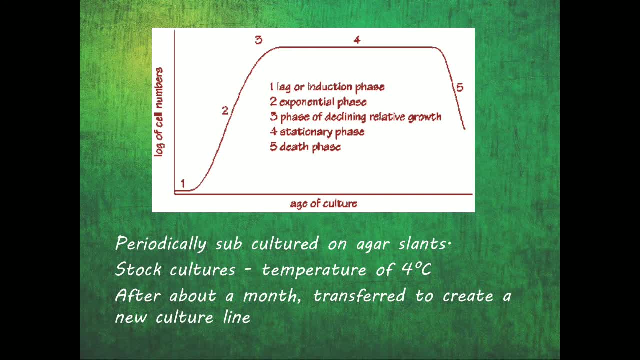 ochromonas. they cannot be stored or they cannot be placed under bright light, because they are light sensitive algae and they will get affected by high light intensity. So these algae need to be kept at very, very low light intensity, maybe about around lesser than 1000 lux, and there 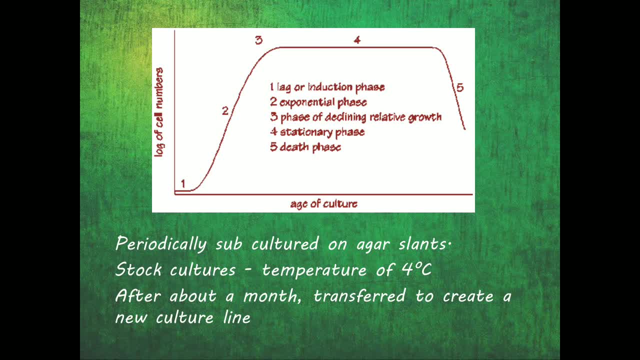 are other algae, such as all the red algae except for forphyridium, all the other red algae, the brown algae and even many of the macrophytic marine green algae. they grow well in dimly lit area of the culture room, So they need not be kept at very high light intensities. This holds good for. 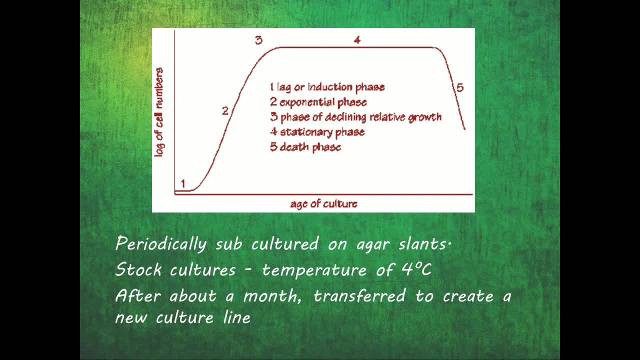 maintenance as well as growth. They can be kept in dimly lit areas and still we are not going to see algae will survive over there. So these pointers about light intensity have to be kept in mind when we are looking for the maintenance of algae. It has to be made sure when we say it. 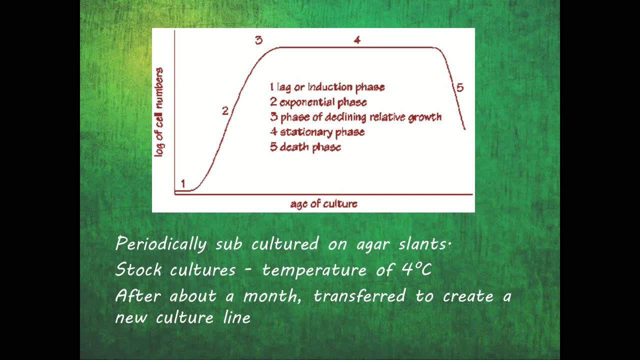 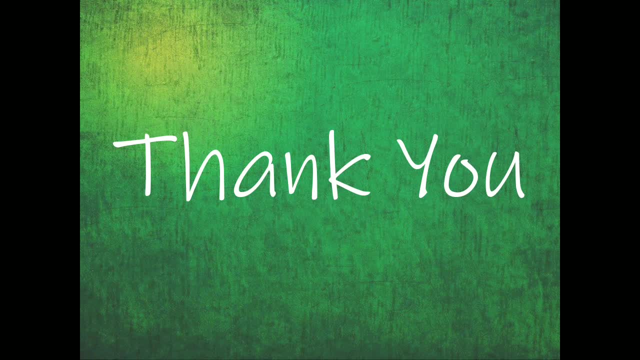 is maintenance. we have to make sure that the algae survive, but they do not grow actively. So these are the different methods of isolation of algae, wherein we have looked into the sampling, that is, the collection of sample from soil and water, the study of various physicochemical 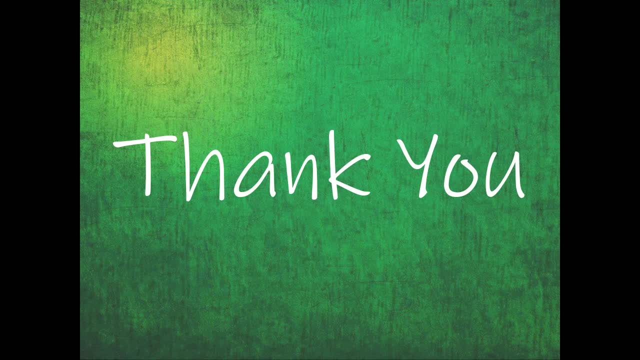 attributes: enrichment of the sample, purification of the sample and finally, the maintenance of the sample. These are the stages for isolation of algae from any environment. Here we have spoken about soil and water, but the methods hold good for any environment. In the next lecture we will see.